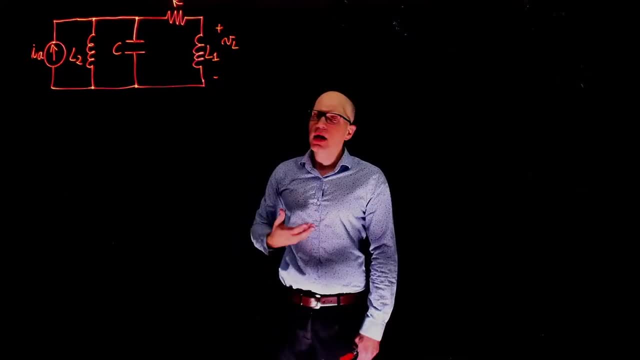 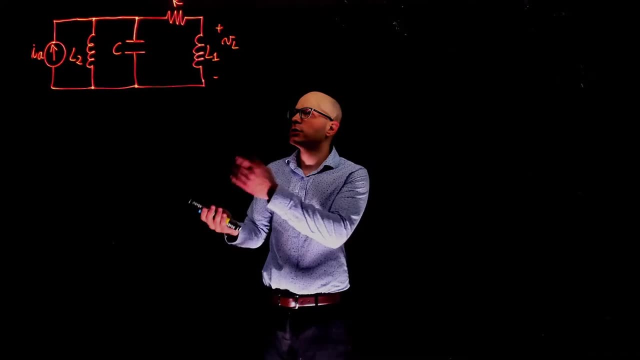 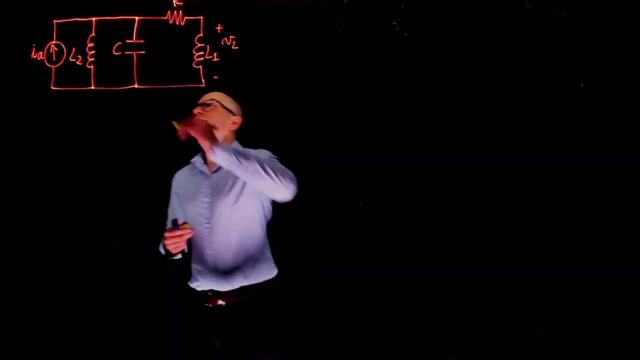 energy in the form of an electrical field and that energy depends on the voltage across that capacitor. So a good choice for the state variables would be the current through these inductors and the voltage across the capacitor. So let's define now the current through the inductor. here let's call this I2.. 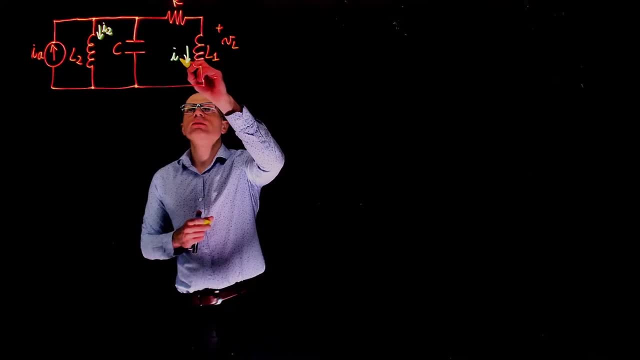 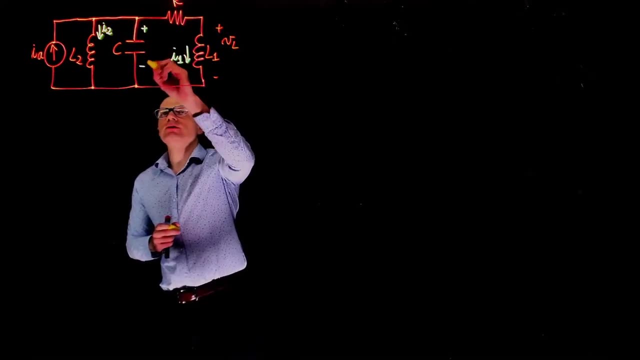 Let's call the current through this inductor here I1,, this is L1, so I1, L2, I2.. Let's call the voltage across this capacitor Vc, And let's define the current through the capacitor as Ic pointing downwards. 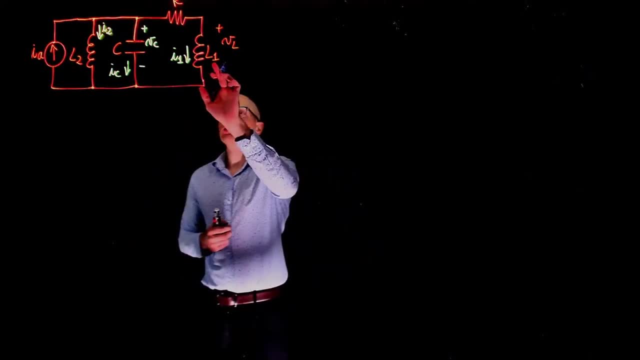 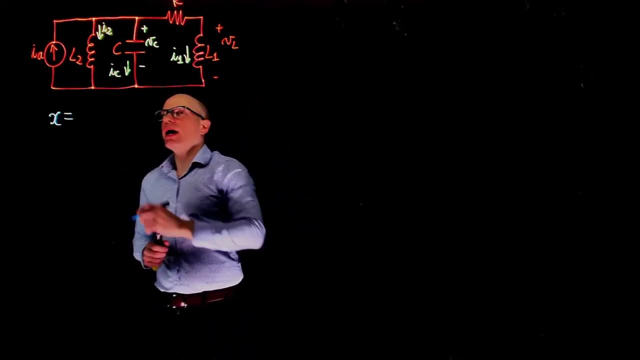 We can now define our state variables as the current through the inductor here and there and the voltage across the capacitor. Let's call our state variables x and you're going to call. then, going this way, the first element here is I2.. 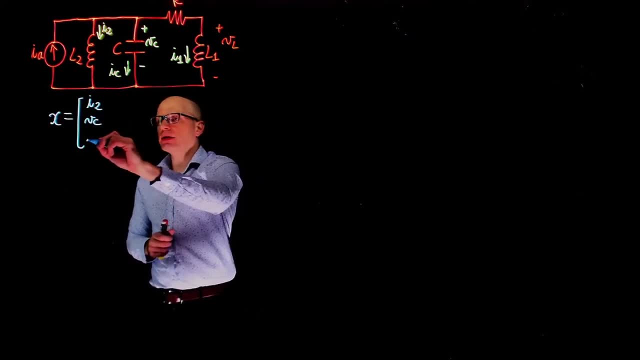 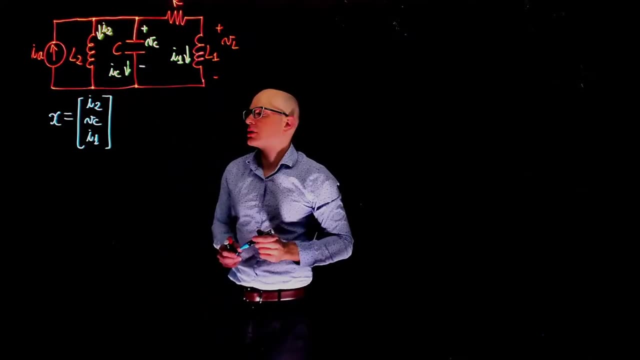 The second element is Vc. Let's call this Vc. And the last element is I1.. The current across this inductor, the voltage across this capacitor and the current across the other inductor. Very well, The first step is done. 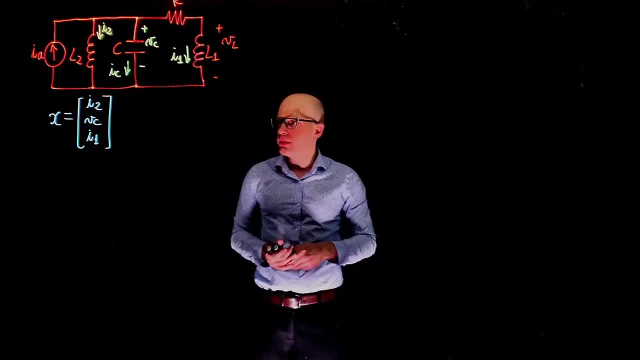 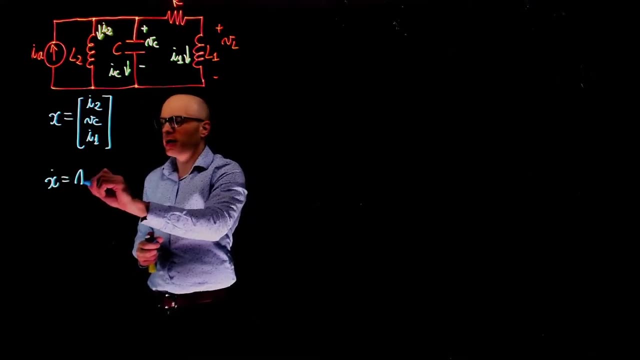 Now we need to find equations for the derivative of these states. Remember that we're looking for the state-space representation, and this will be done in the form of x equals, dot equals to Ax plus V times U. U is the input which, in this case, 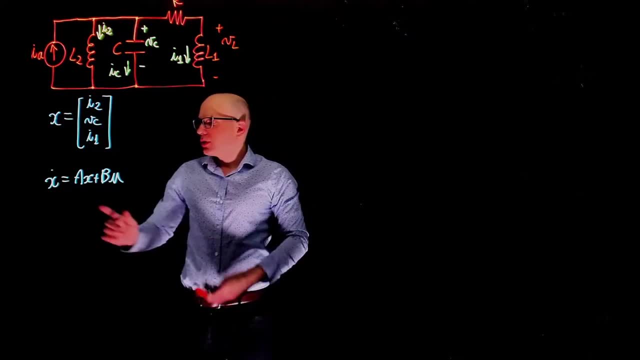 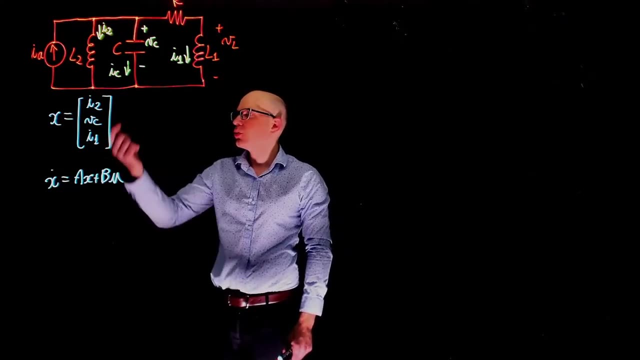 is Ia. What do we see here? We see x dot, which is a function of x itself. So we now need to come up with three equations: one for I2,, one for Vc, one for I1, that will. 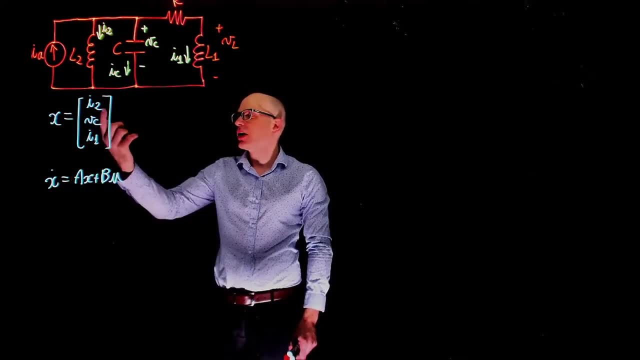 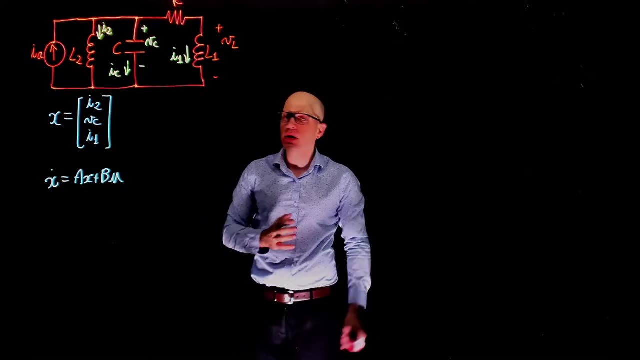 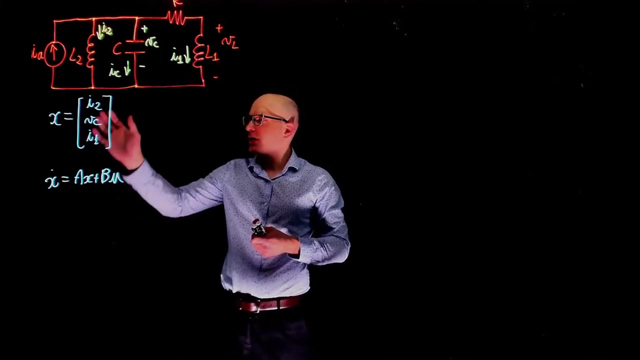 follow this format: where you have the derivative of I2 will be a function of all other states, The derivative of Vc a function of all states, the derivative I1, a function of all the other states, And it is also important to note that these equations will be the derivative of Vc in 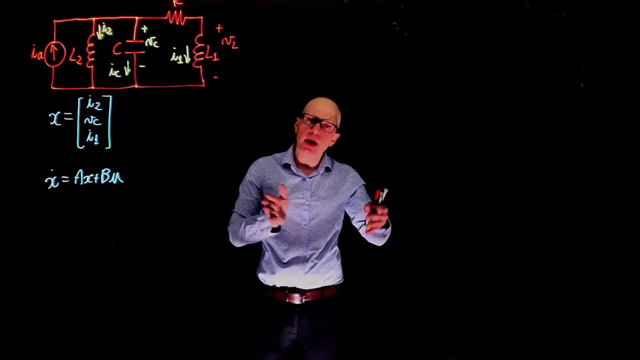 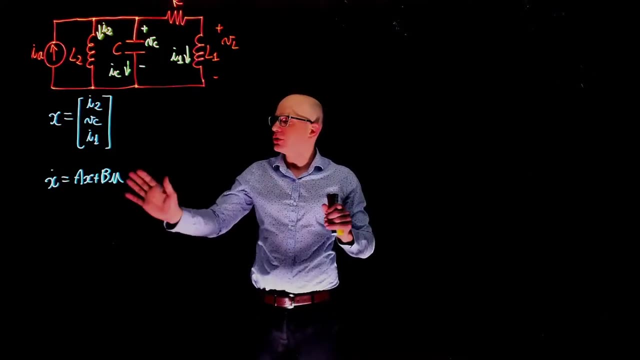 this case, derivative of these state variables. they only depend on the states. they do not depend on the derivative of the states. so we need to also ensure that the equations that are going to develop now will follow the same format as here, so that will make everything easier than when we have to put 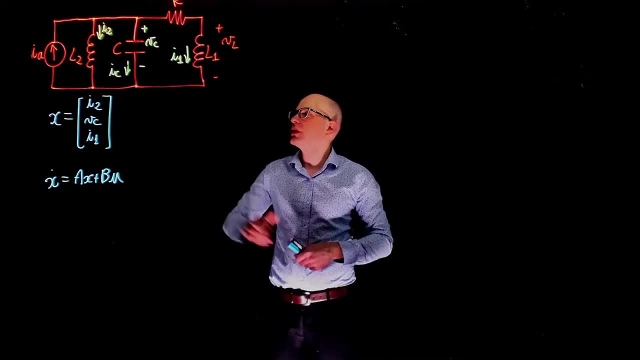 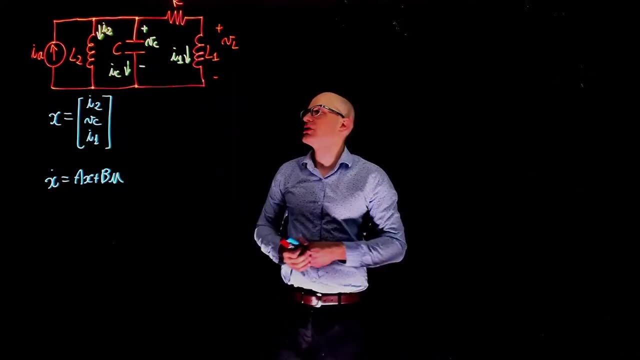 everything in a matrix form. okay, so let's start now. let's start by looking for a equation that gives us the derivative of the first state, i2, as a function of other states. what can we conclude here? can we somehow link i2 and vc, for example? or can we link i2 and i1 and vc? 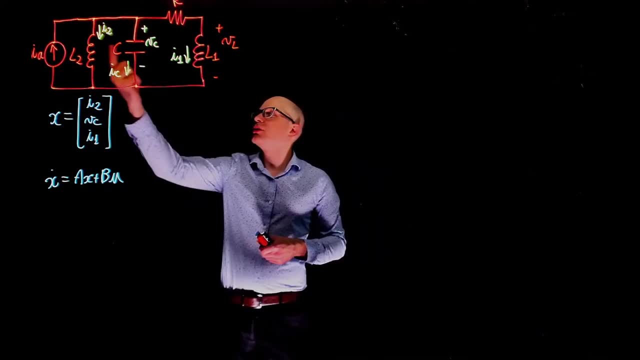 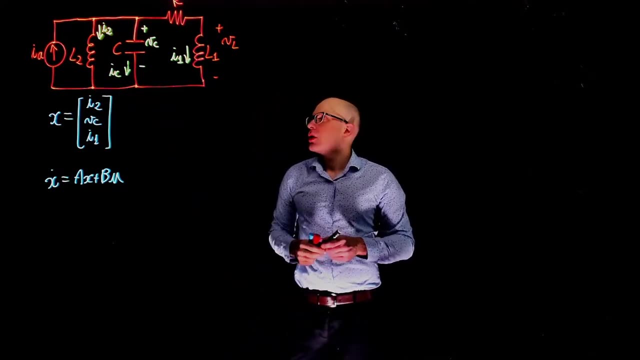 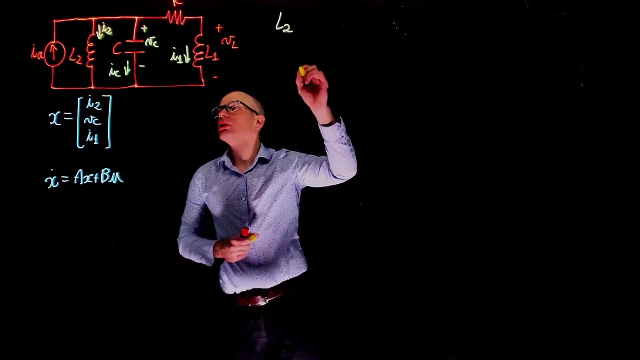 well, clearly it would be easy here to link i2 and vc, because the voltage across the inductor and the voltage across the capacitor are exactly the same. what is the voltage across the inductor? the voltage across the inductor l2 is l2, d, i, 2. 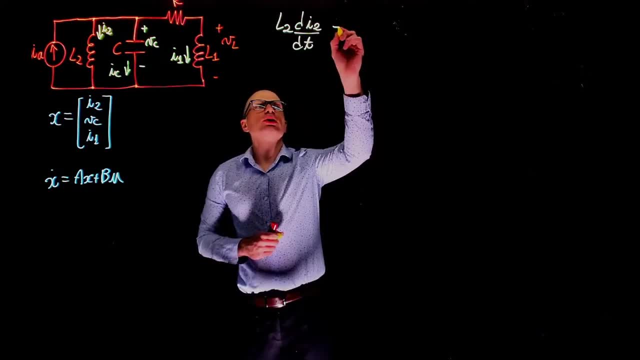 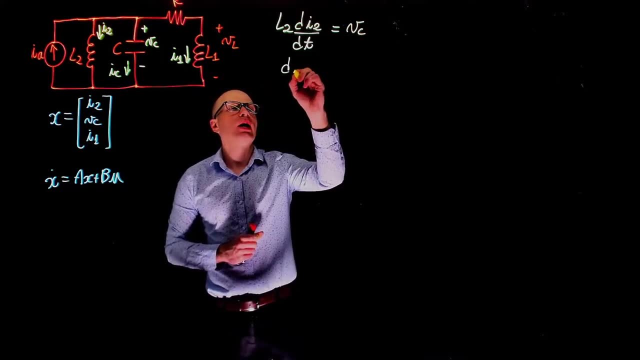 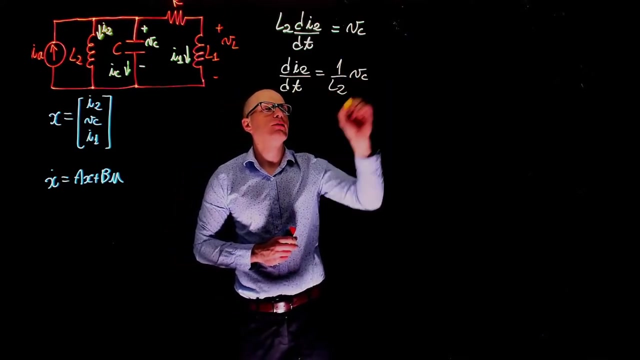 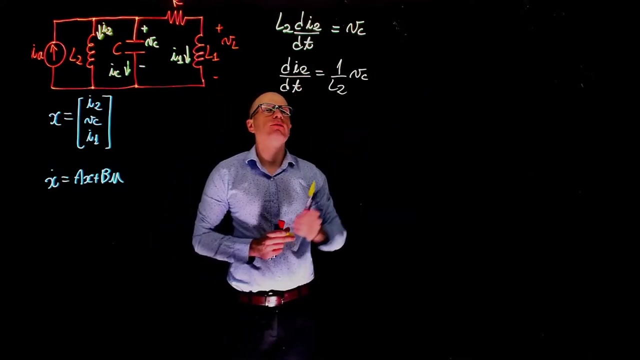 dt and the voltage across the capacitor is simply vc. couldn't be easier than that. now we have di2 over dt equals to 1 over l2 times vc. here we have the expression we need for i2. i2, the derivative of i2, is a function of other states. if we call this vector here, 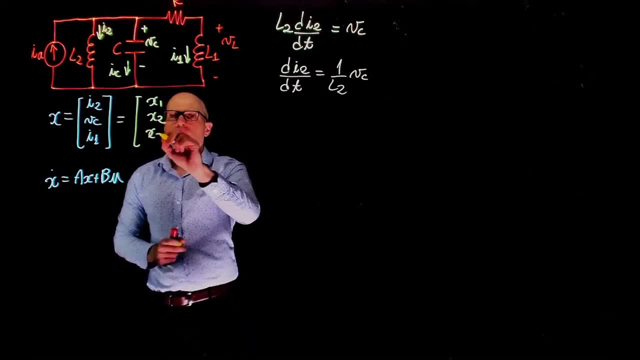 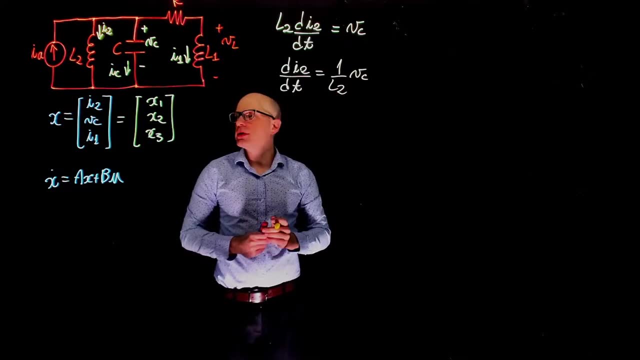 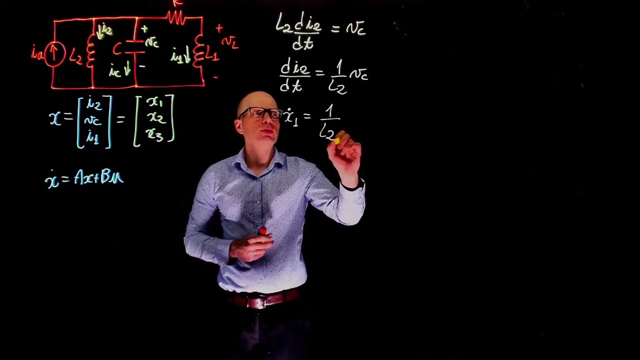 x1, x2 and x3. so i2 is x1, vc is x2, i1 is x3. how can you rewrite this expression now? we have x1, dot equals to 1 over l2 times vc. vc becomes x2, and here we have the first equation. 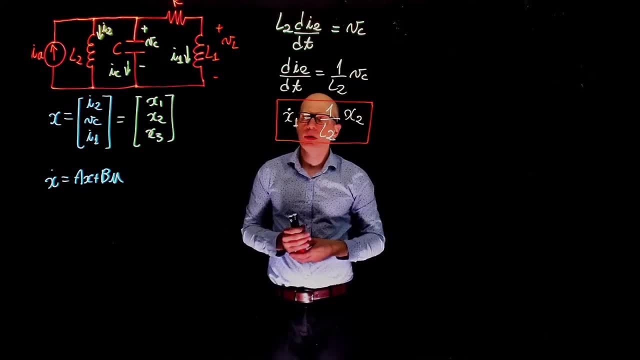 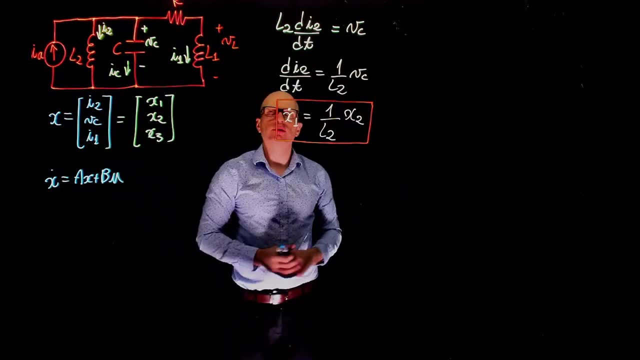 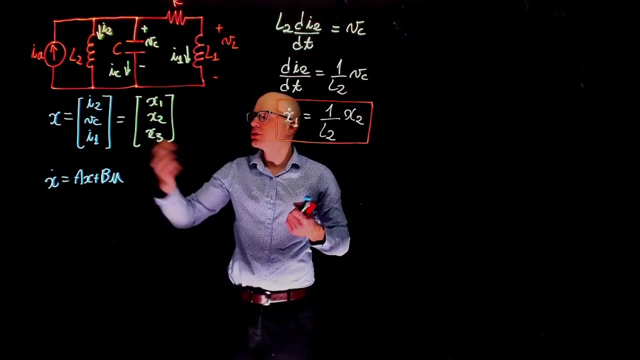 needed for this manipulation. now let's look at vc. we need a similar expression. we need the derivative of vc equals to a function of other states. now let's think about this problem. we want something that depends on the derivative of vc because that's one of our states. what is that? what is something? 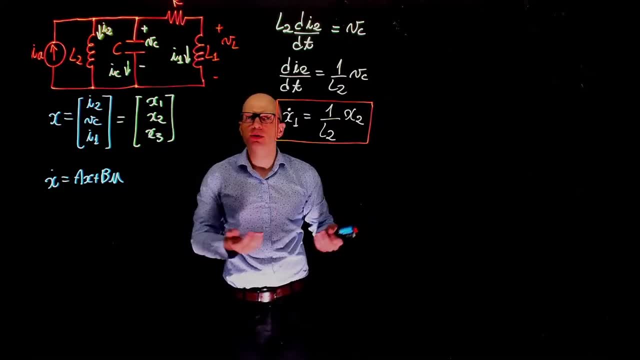 that is proportional to the derivative of a voltage in a capacitor. well, that's the current through the capacitor. so let's now relate ic and vc. ic is not one of our states, vc is. we can write that the current through this capacitor, ic, is c times, dv, c, dt, aha. 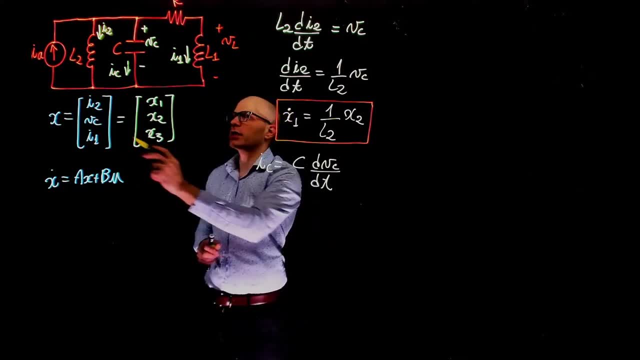 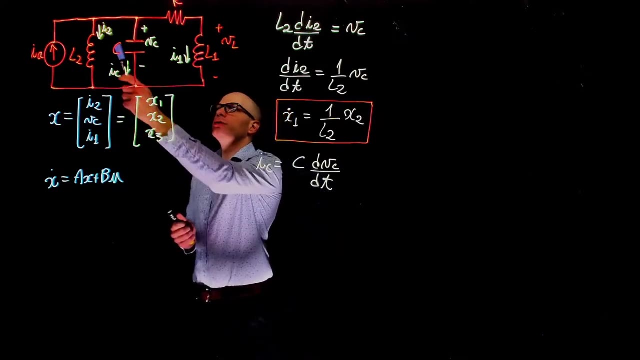 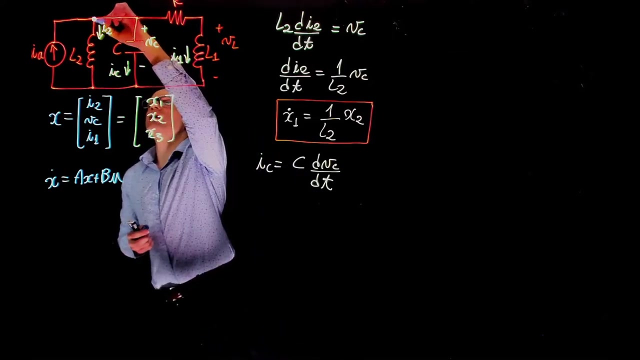 here is the derivative of vc, the derivative of the second state. now, what is ic? ic is not one of our states we need to get rid of. it is an internal variable we can relate ic with to i2, to i1 and to the input ia. that's easy. we can just look at the current at this node, a here. 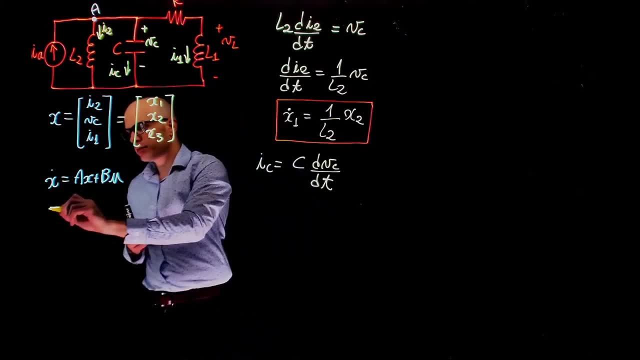 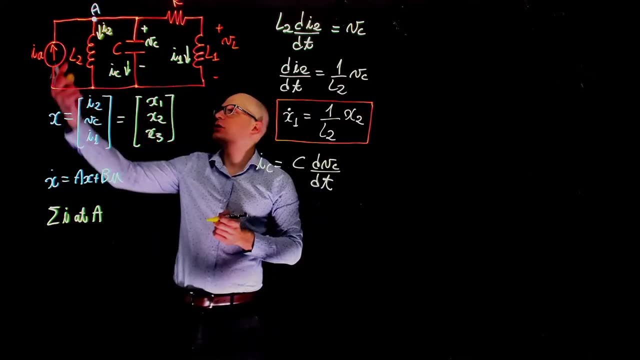 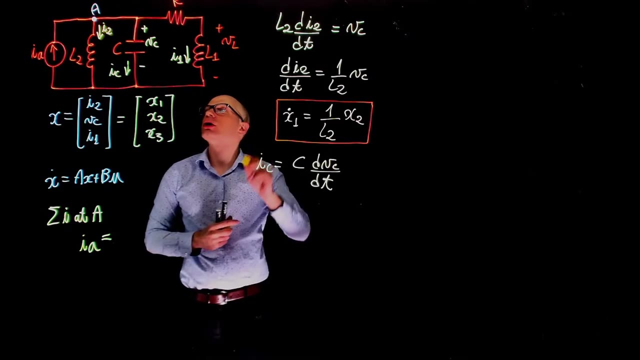 and do the sum of all currents at node a, what do we have? we have the current going in, that is ia, and this is equal to all other currents coming out of that node, that is, i2 plus i1 plus ic. now notice that this equation is very helpful, because the only thing here that 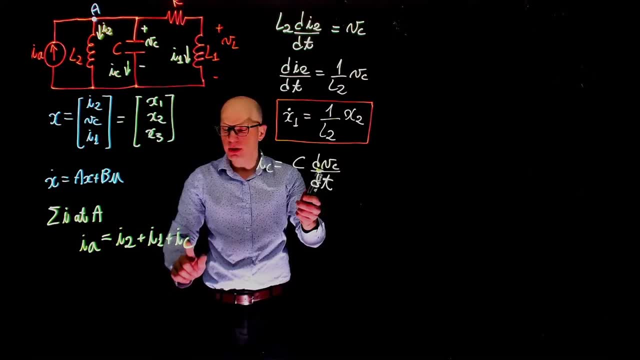 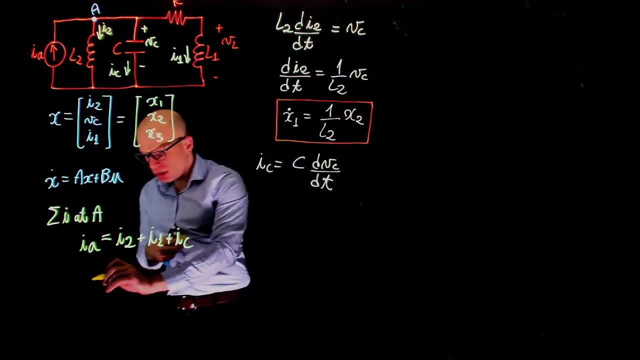 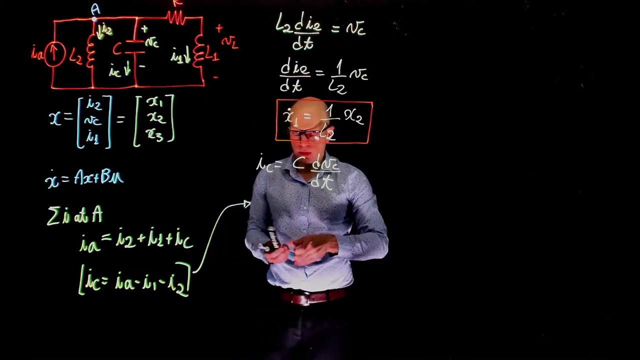 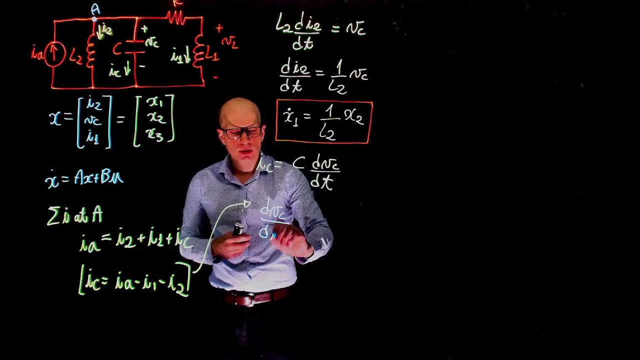 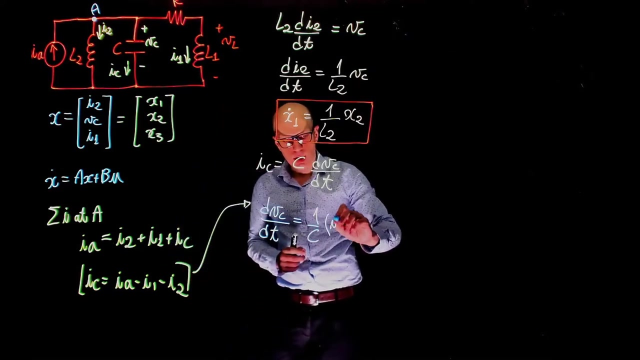 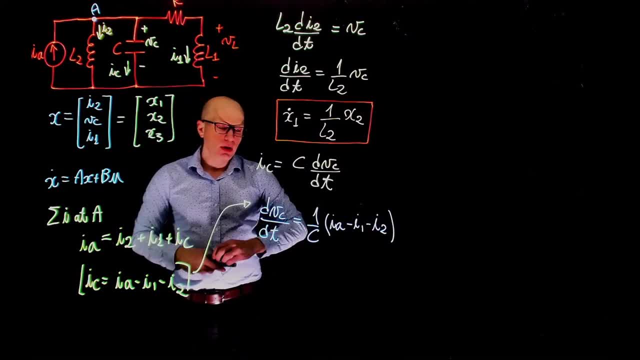 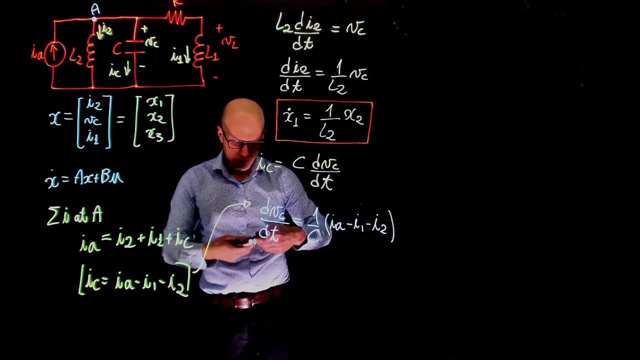 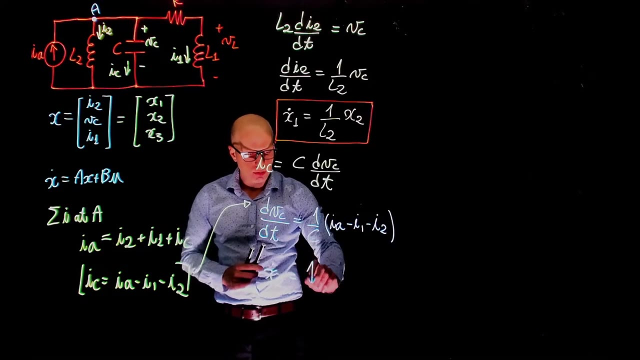 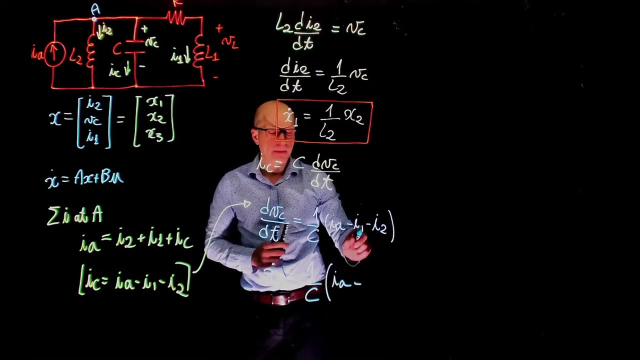 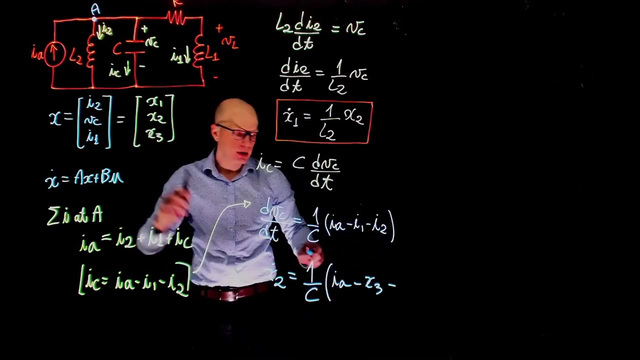 using the state space representation. here DVC DT becomes X 2 dot because VC is X 2. so this is X, this is X 2 dot 1 over C is a constant. I a is an input, don't need to change it. I 1 is X 3 and I 2 is X 1. and here we have the second. 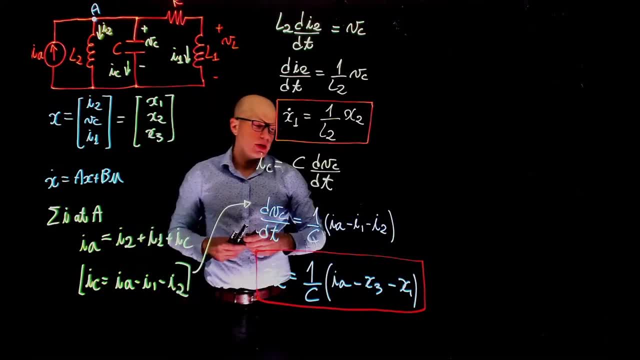 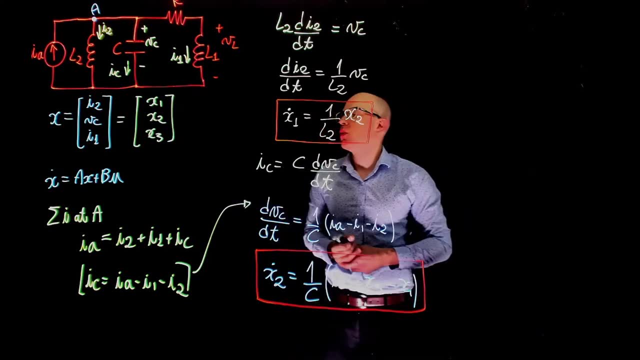 expression for our state space representation. we are missing one equation. now we are looking for a equation for the derivative of I 1 as a function of other states. how can we do that now? we could apply here the derivative of I 1 as a function of other states. how can we do that now? we could apply here. 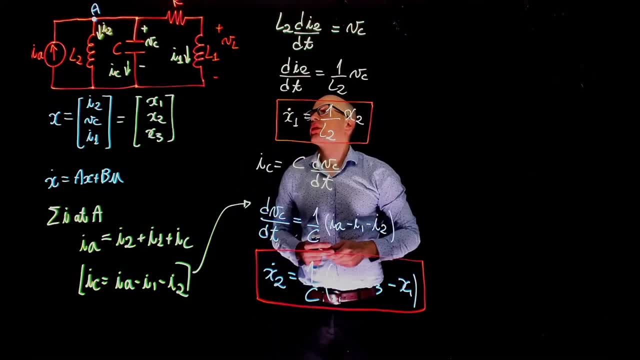 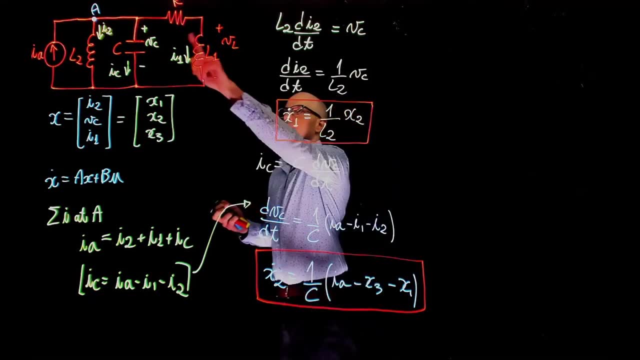 Kirchhoff's law to this loop and do the sum of all voltages there. if you do that, we'll see that at this, voltage across here will be a function of I 1, because that's the voltage across the resistor. will be a function of VC, which. 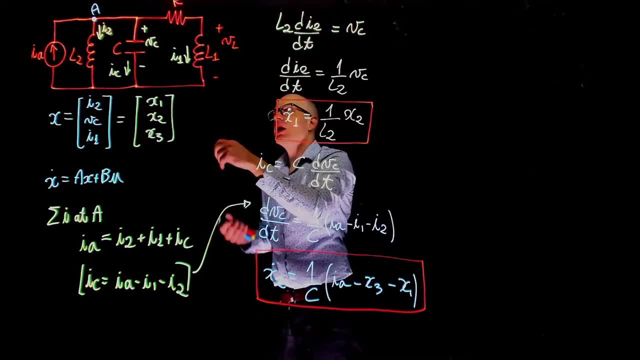 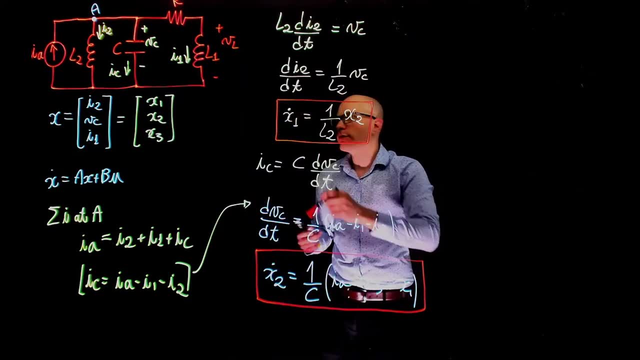 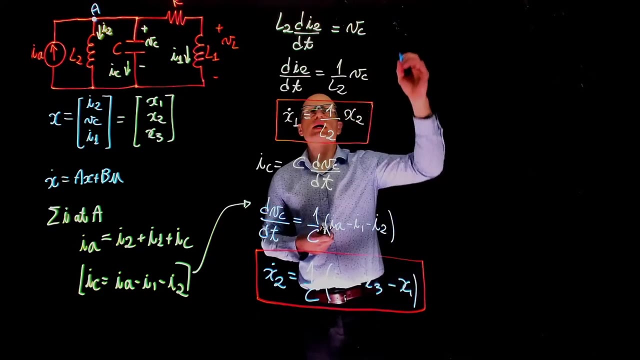 is another state, and this makes things very convenient because the voltage across the inductor is also a function of I 1, a function of one of our states. so if you now do Kirchhoff's law in this loop here, what do you have? we have that R times I 1 plus the voltage. 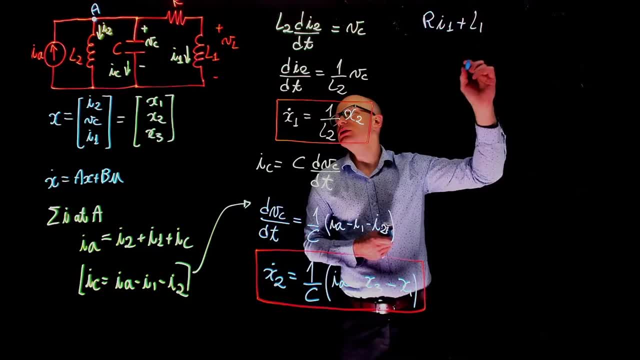 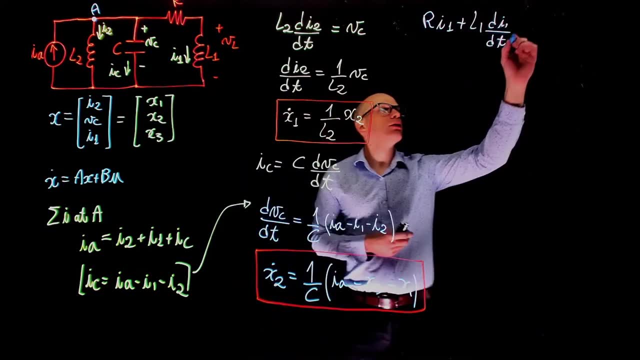 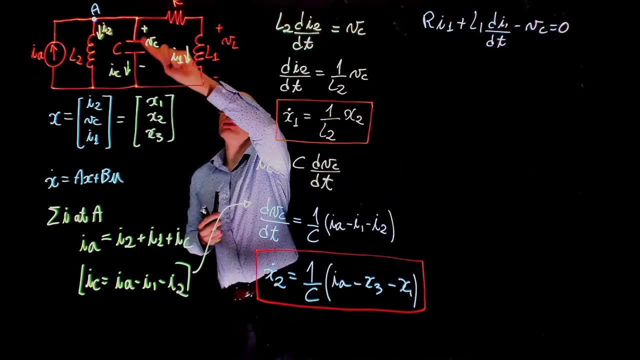 across. this inductor is l1 Di 1 aha. DT minus VC equals to zero. why minus VC? because the current through VC is pointing down. so when you go through, the current through VC is pointing down. so when you go through, the current through VC is pointing down. so when you go 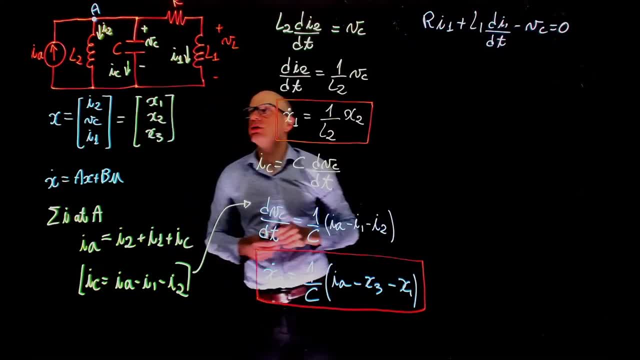 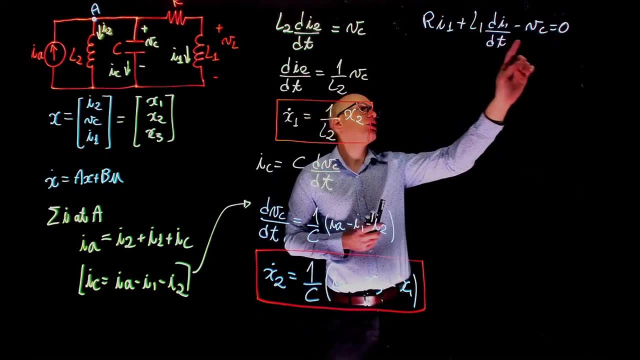 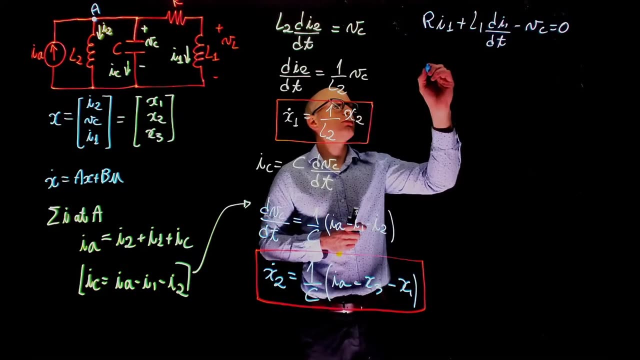 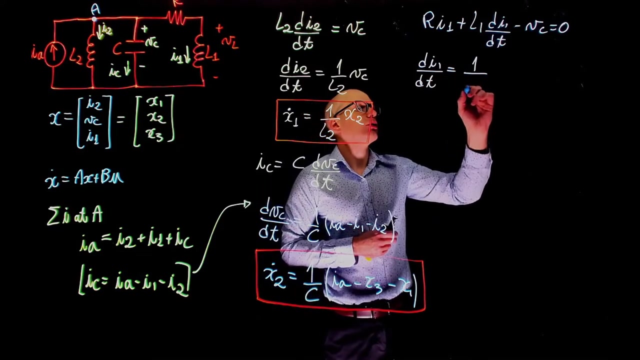 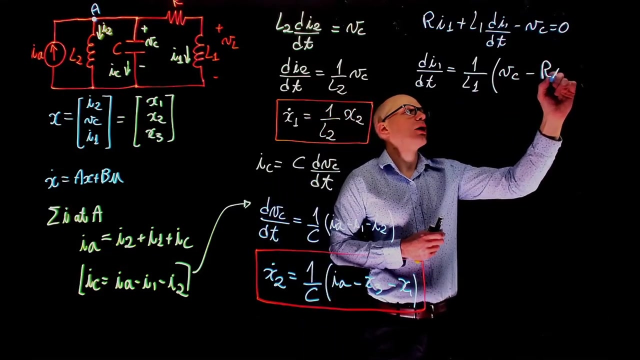 counterclockwise. here we are going against the current through VC, hence the negative sign. This equation is perfect because we have everything here as a function of the states. Now we can isolate DI1DT, and DI1DT is simply 1 over L1 times VC minus RI1.. Now we can write this in the state: 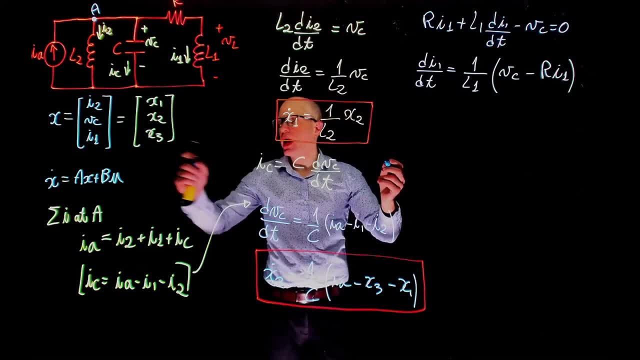 space: DI1DT becomes X3 dot 1 over L1 times VC minus RI1.. Now we can write this in the state space: DI1DT becomes X3 dot 1 over L1 times VC minus RI1.. Now we can write this in the state space: DI1DT becomes X3 dot 1 over L1 times VC minus RI1.. 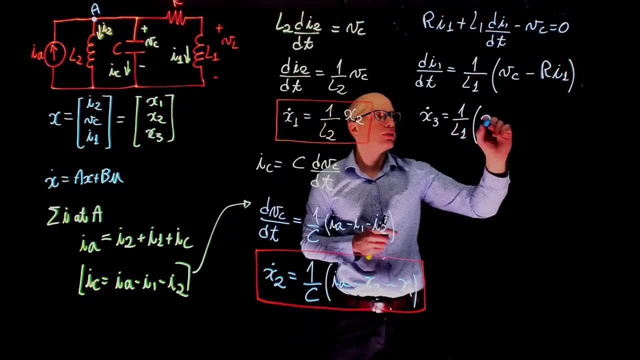 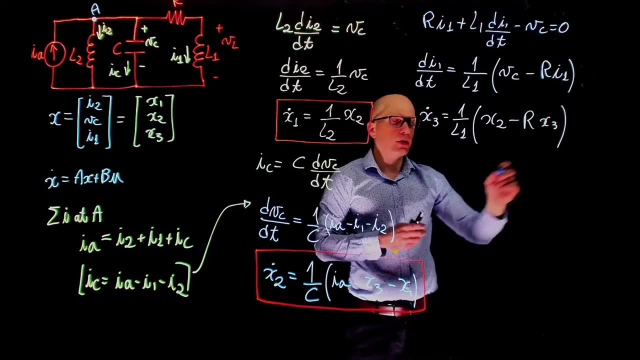 Now we can write this in the state space: DI1DT becomes X3, dot 1 over L1 times VC minus RI1.. VC is X2 minus R times I1, which is X3.. Here we have the third expression for our circuit. 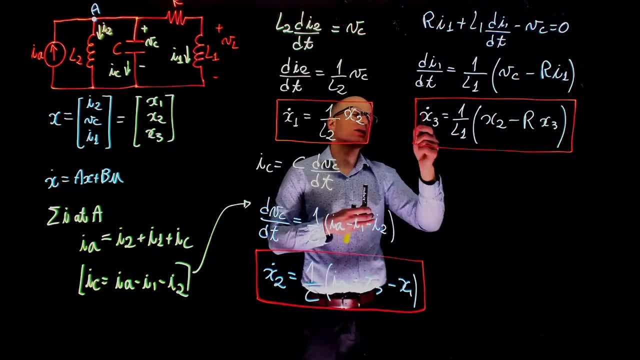 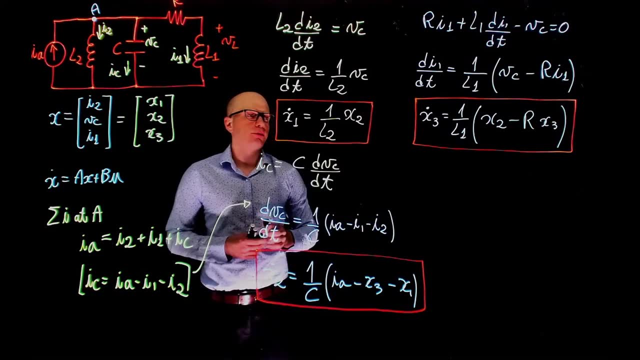 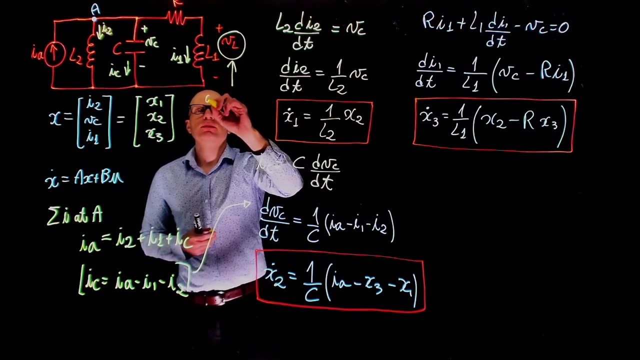 Third state, represented as a function. the third state, derivative, represented as a function of other states. All right, now we have these three expressions, we need to define our output. Our output here is VL: is the voltage across this inductor. Now we need an expression for the output as well. Let's write it here. 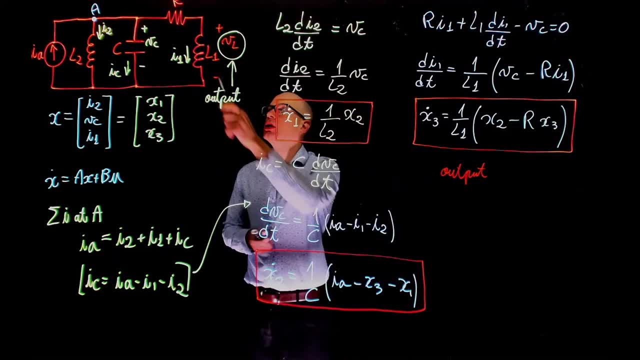 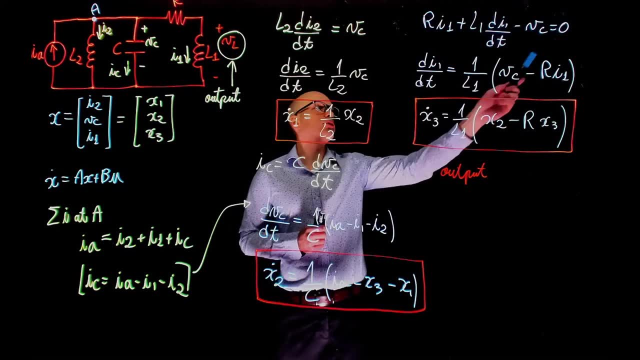 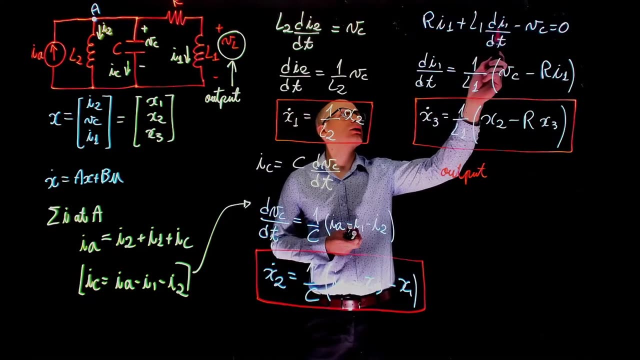 How do we find that one? We want the output to be a function of the states, not the derivative of the states, just the states. Well, we can actually do the same Kirchhoff's law that we did here. The exact same, but instead of writing L1, DI1DT. this whole thing here is, in fact, 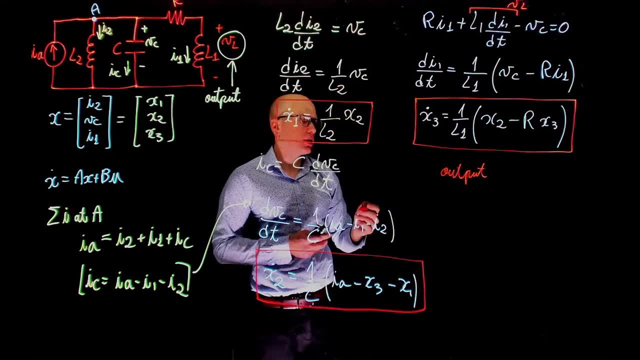 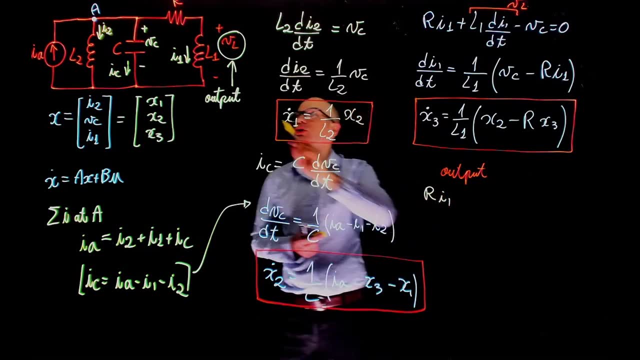 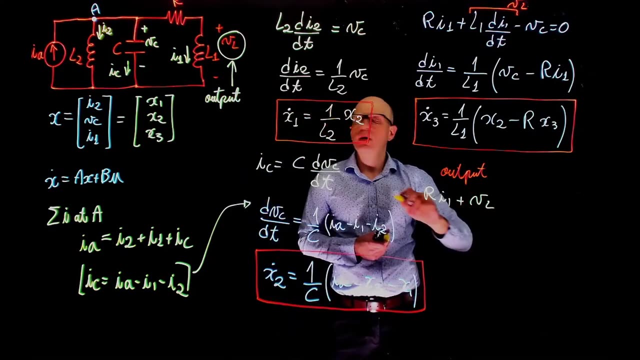 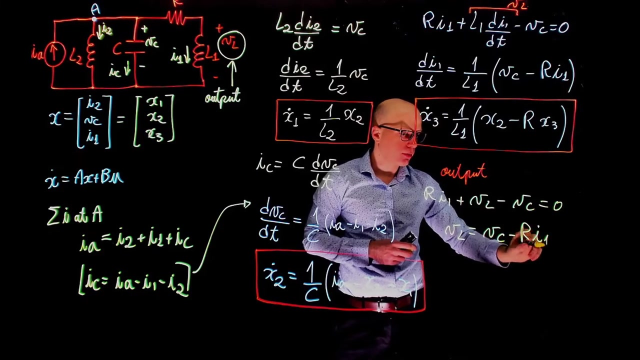 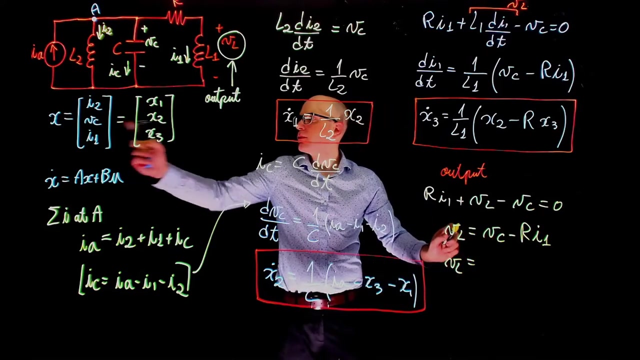 VL is the output, So we can reuse that expression and rewrite this as RI1, the voltage across the resistor plus the voltage across the inductor. VL minus VC equals to 0.. So VL, the output, becomes VC minus RI1. in state space, or using the state space variables, we have VL equals to VC, X2 minus R times I1, which is X2.. 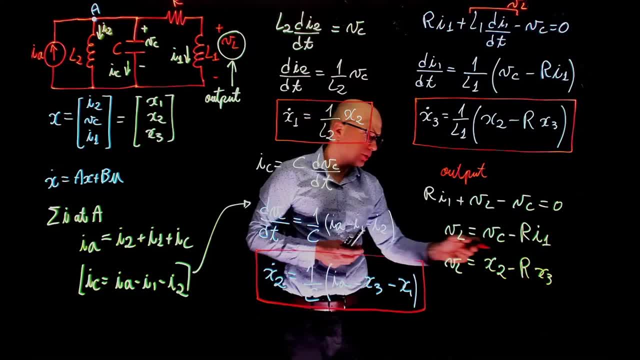 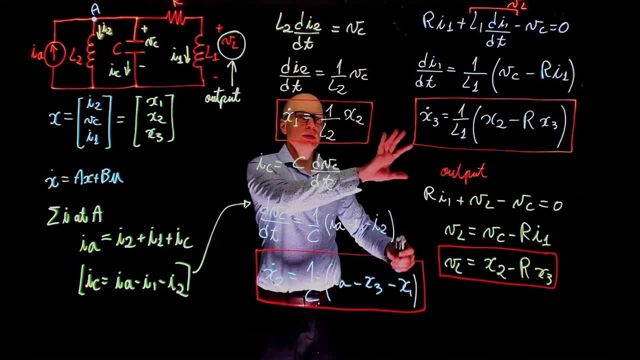 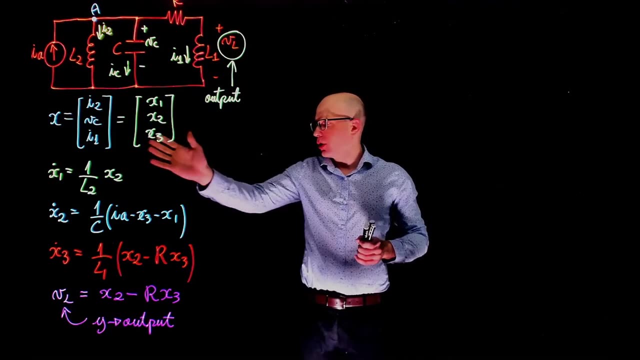 And there it is. That's the expression for the output. Now that we have that, I'm going to erase everything, save these equations, and you're going to represent them in a matrix format. Very well, so here we are with all the expressions we. 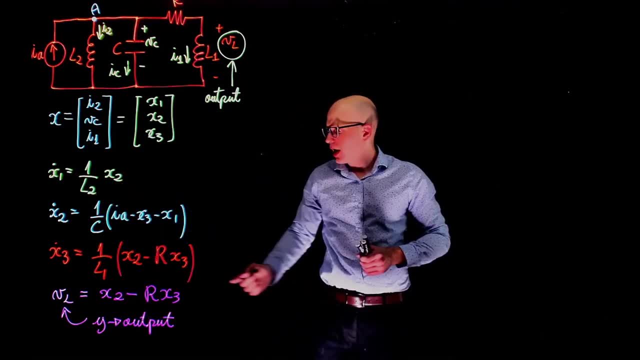 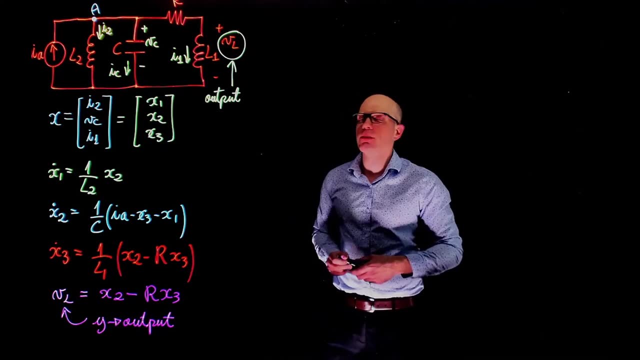 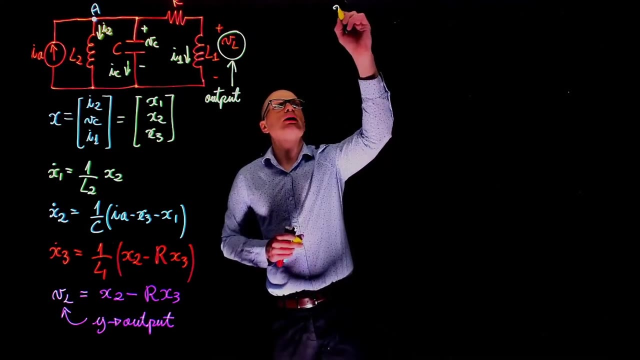 derived before: X1 dot, X2 and X3 dot and VL, the output, The output which is VL, that is the same as Y in the standard form for state space. Now let's write these equations in the standard state space representation. The first one will be: X dot equals to A times X plus B times U. U is the input to the system, which is: 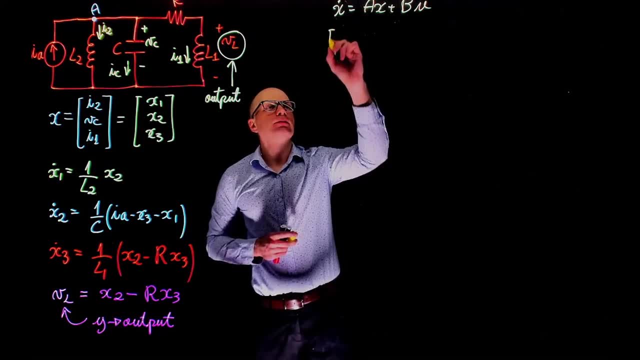 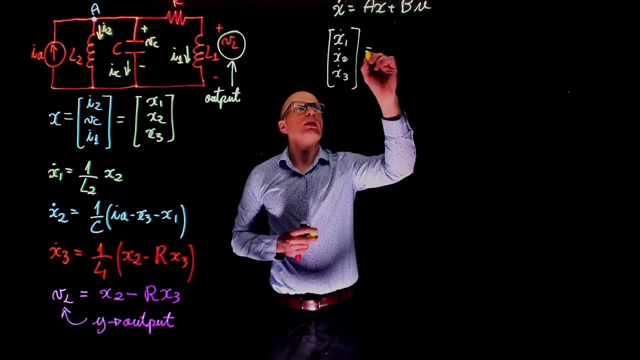 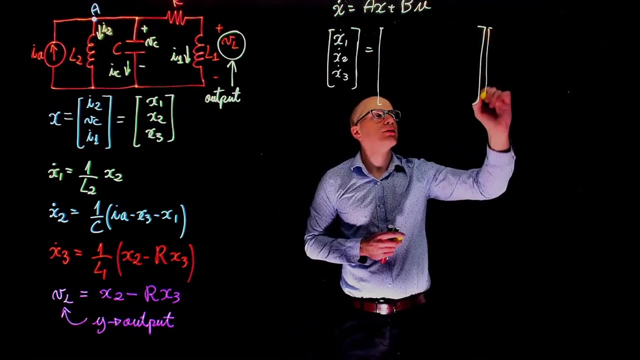 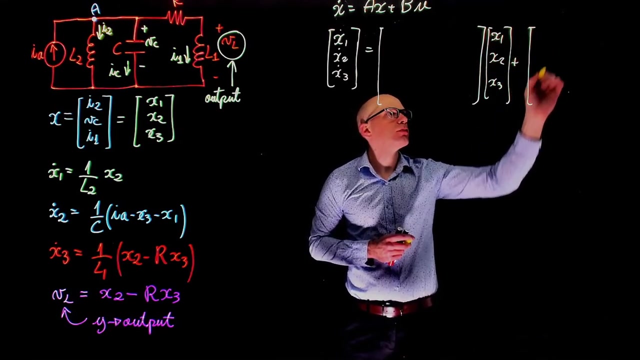 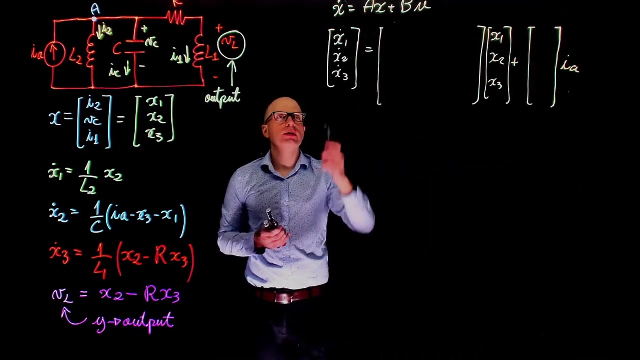 IA. X dot is X1 dot, X2 dot, X3 dot is A times X, X1, X2, X3 plus B times U, which is IA. What goes in there? So let's look at X1 dot For X1 dot. we're looking at this expression here. 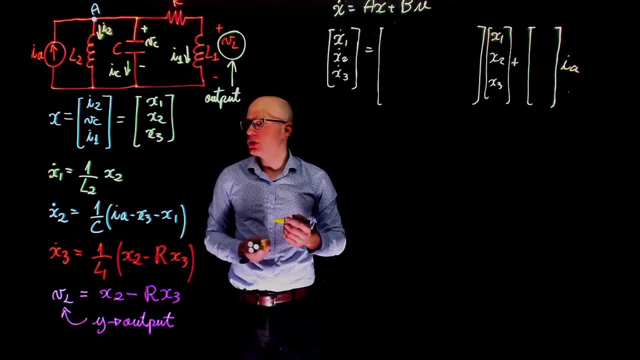 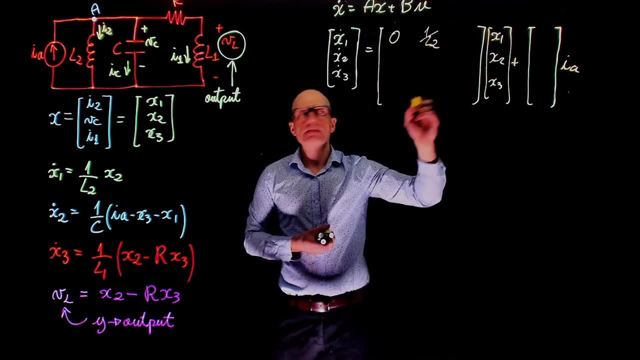 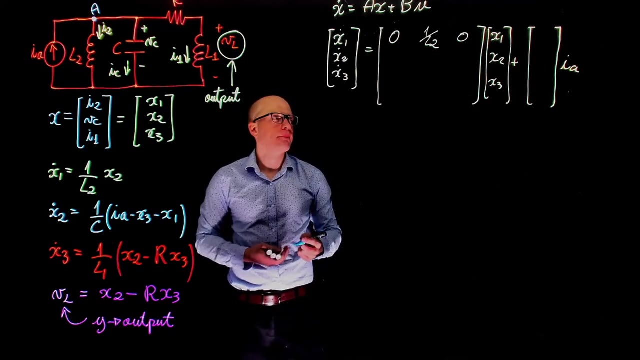 X1 dot only depends on X2 and has this coefficient 1 over L2.. So this is 0, 1 over L2, 0, 1 over L2 zero. now let's look at x2 dot. x2 dot depends on the input, depends on x3 and x1. so we have 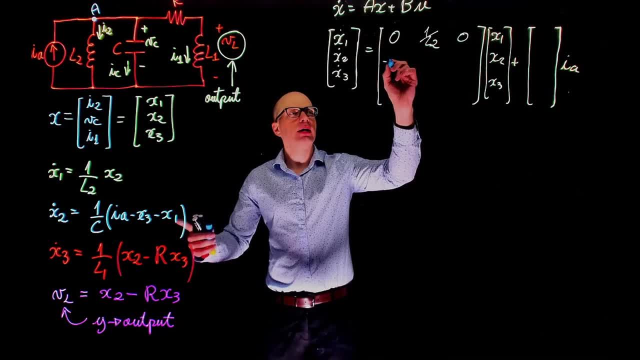 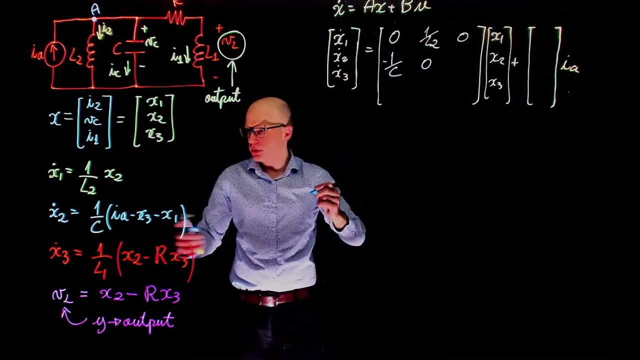 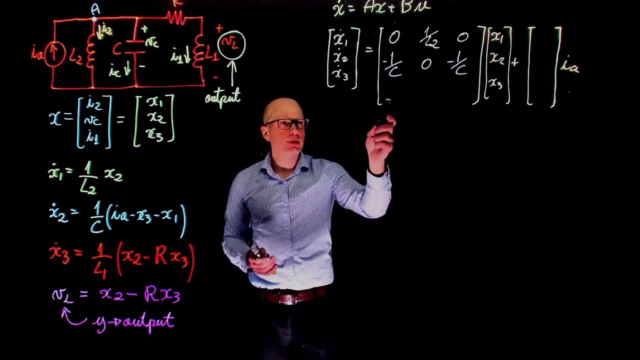 for x3. for x1 we have negative 1 over C, x2 is 0 and x3 is also negative 1 over C. we'll do the output later. so long let's complete the third row here. that's for x, 3 dots and this depends on x2 and x3. so there is no x1. this is 0 for x2 we have. 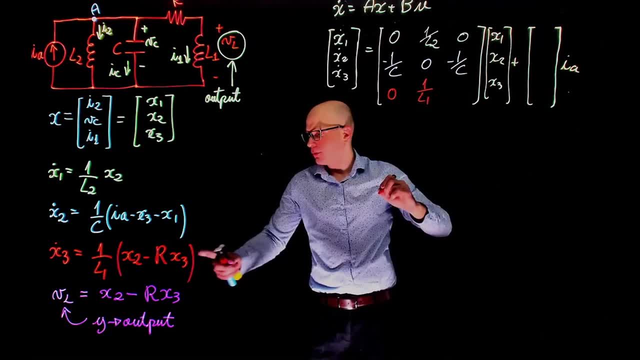 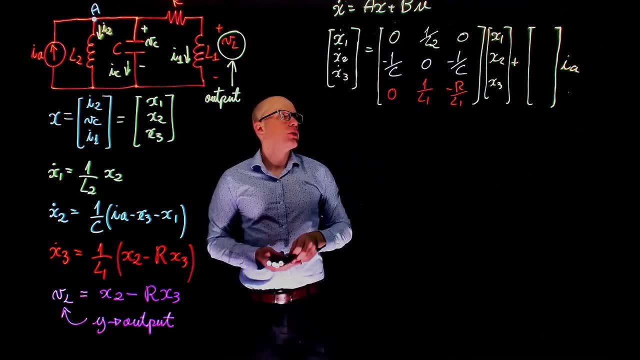 x1 and x3. so we have negative 1 over C and x2 is 0, and x3 is also negative 1 over C. so there is no x1. this is 0. for x2 we have 1 over L 1 and for x3 we have negative R over L 1. now let's look at the input. 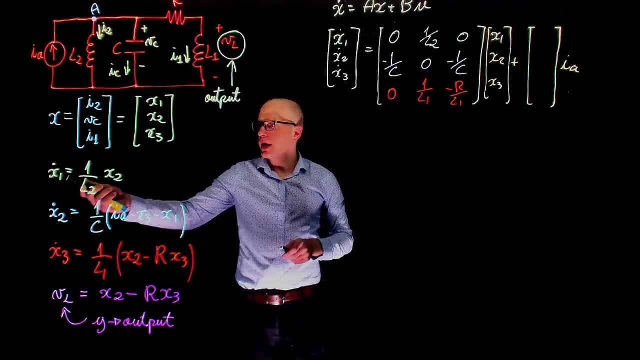 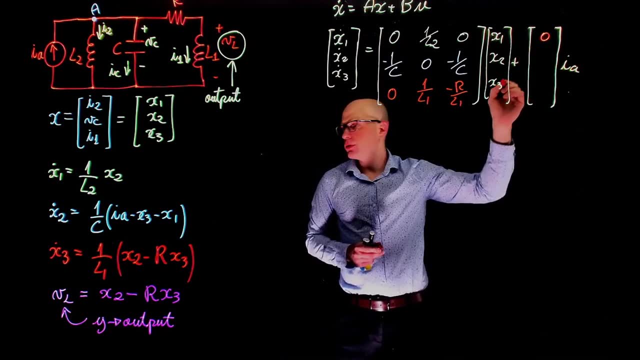 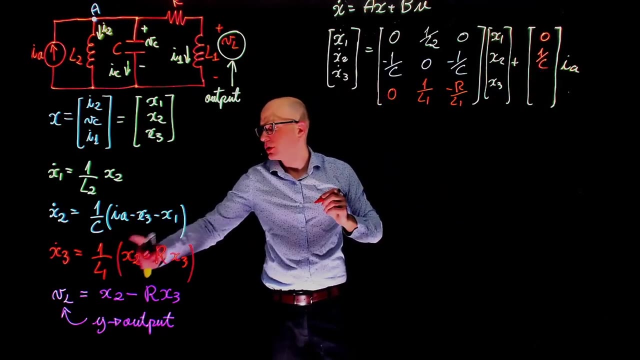 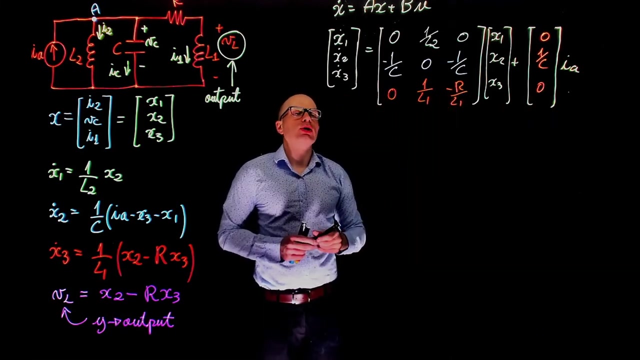 the input doesn't show in x1 dot, does only shows in x2 dot. so for x1 dot we have 0, for x2 dot we have 1 over C. I will show here for this part of the equation. and for x3 dot we have 0. okay, so this is our first equation. now we need